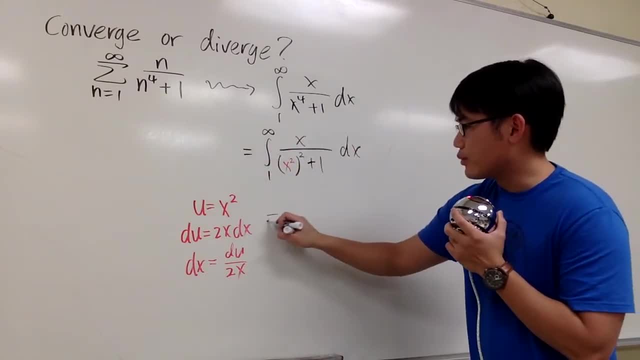 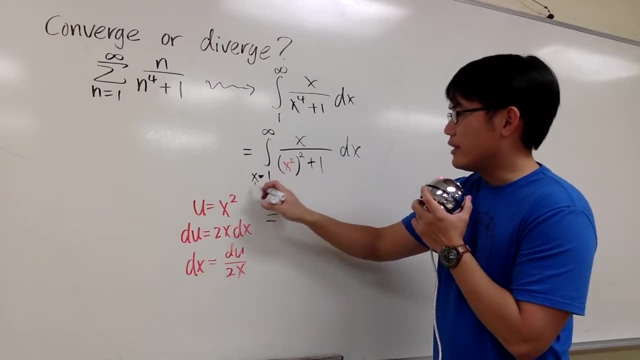 So let's take this integral into the u-world, So I will put this down right here. Well, we also have to change the number, right? So let's see, This is 1, and that's Actually when x goes from 1, right, this is the number in the x-world. 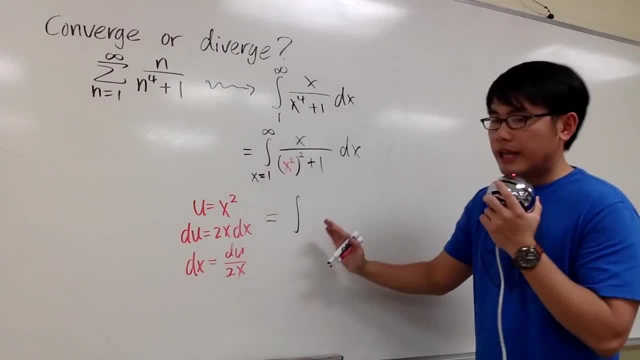 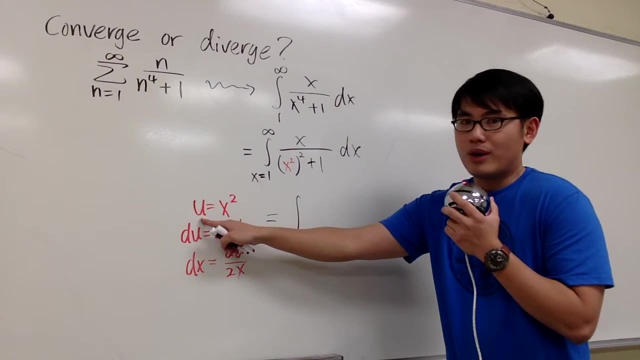 x goes from 1 to infinity. But then, if I want to take this into the u-world, when x is 1, we put the x right here: 1 squared, which is just 1, and that's the same as u is equal to 1.. 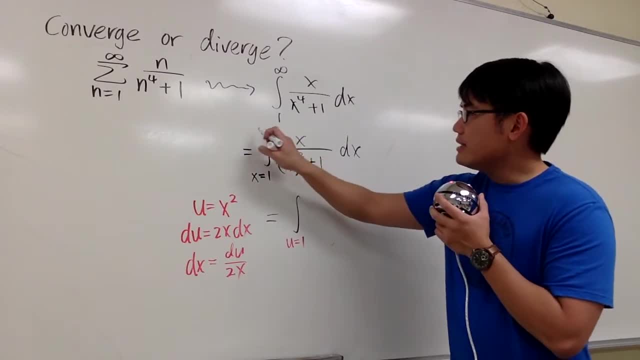 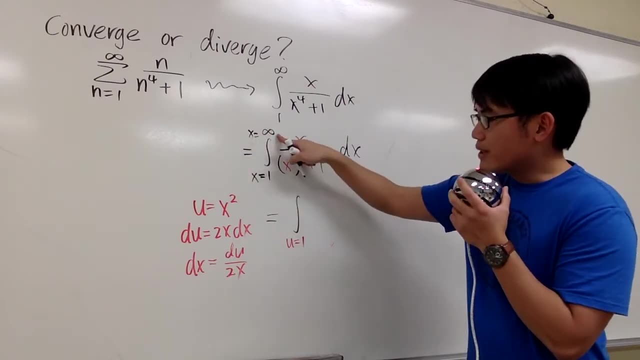 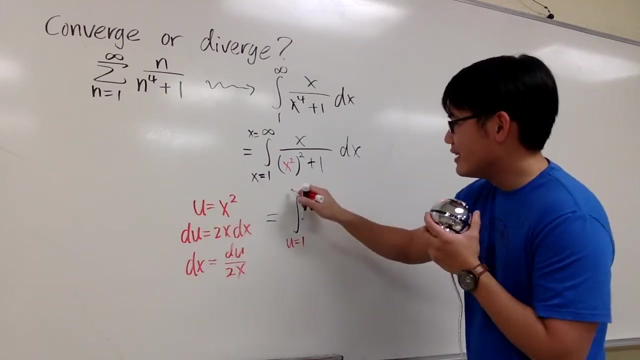 u will be 1.. And then if x was infinity? let me just write this nicely right here, okay, Okay, See, put the infinity right here. Infinity squared. we still have infinity. Therefore u is also infinity. So we are still trying to, you know, change the limits of integrations, but in this case, 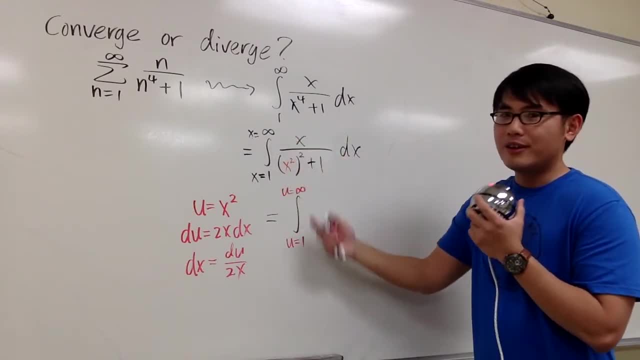 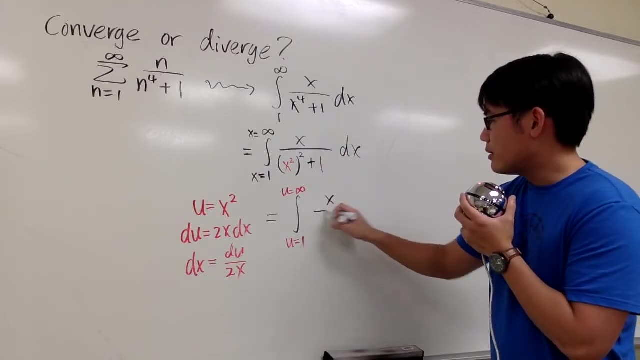 it happens to be the same as the original. 1 to infinity here, 1 to infinity here. But then you have to do this very carefully, okay? And then the x is still on the top. Let me just put that down. 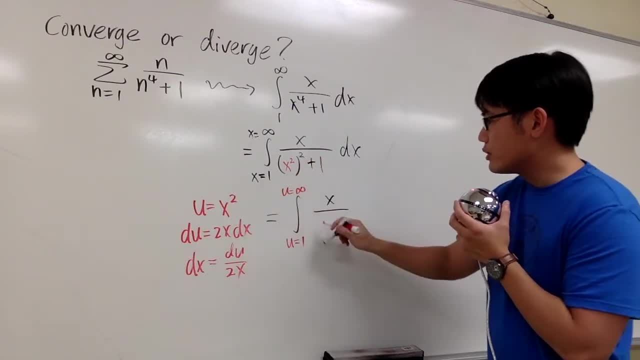 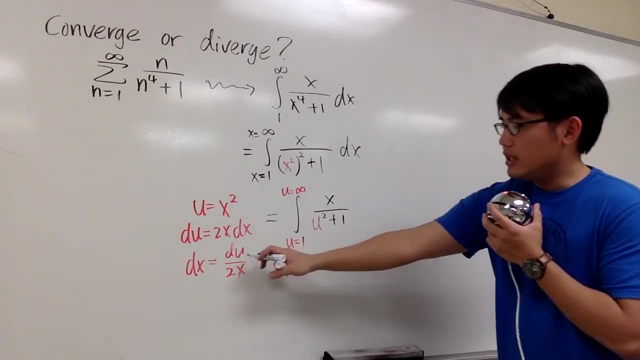 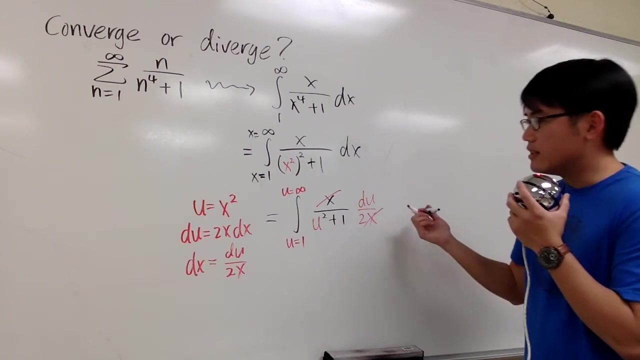 Over the x squared in red, it's u, So we have u squared, and then plus 1.. And then the dx is du over 2x. So let me put this down: du over 2x. And, as we can see, this x and that x cancel each other out. 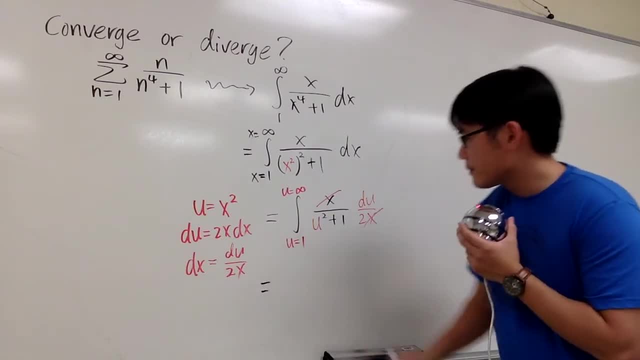 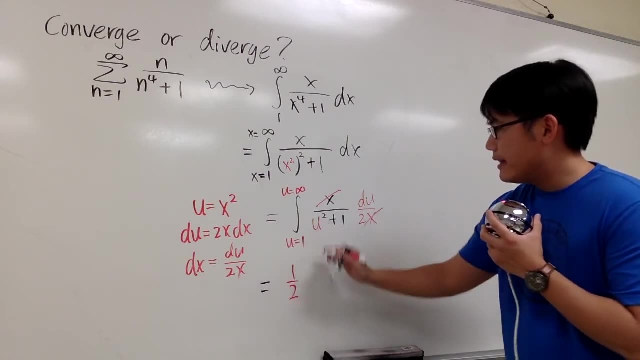 And now let's just work in the u-world. So let's see how do we get. We have 1 over 2.. Let's take that outside of the integral, So we have 1 over 2. And then the integral in terms of u will be going from 1 to infinity. 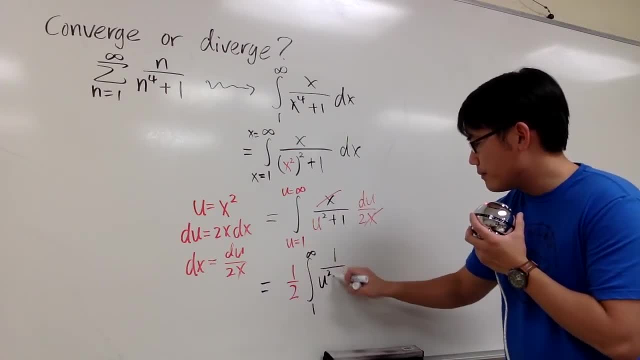 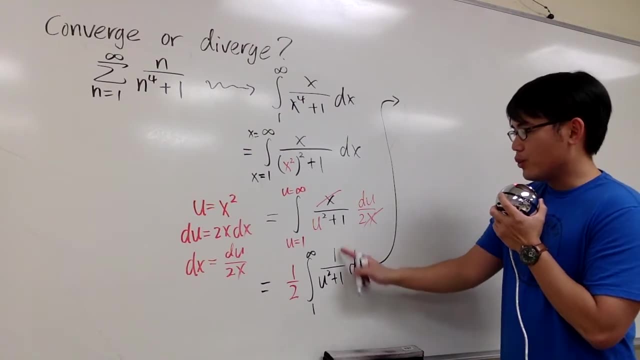 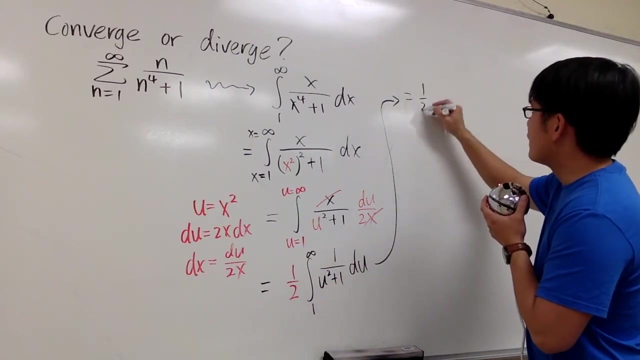 And then this is 1 over u squared Plus 1 du. All right, So how are we going to integrate this 1 over u squared plus 1.. This is just inverse tangent. So we know this is going to be equal to 1 half times the inverse tangent. 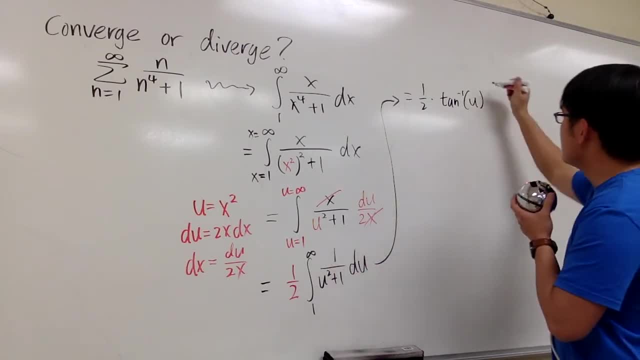 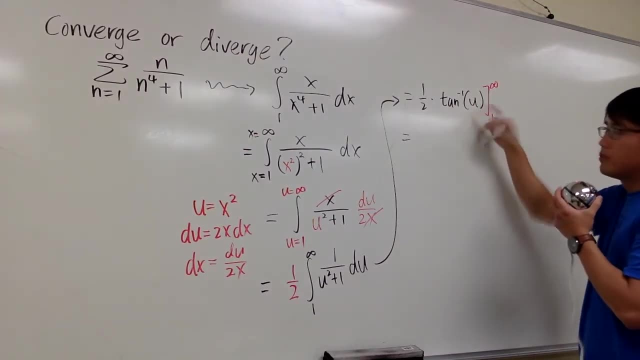 And this is in the u-world And it goes from 1 to infinity. So let me put this down as 1 to infinity And plug in infinity into u, first Subtract. plug in 1 into u. Okay, And let me just put down the 1 half. 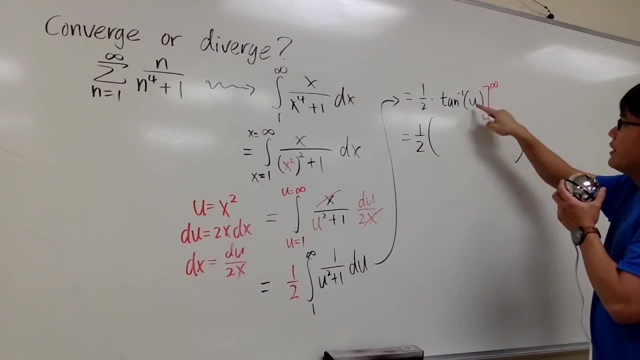 All the way to the front And open the parentheses, Put the infinity right here, So we have inverse tangent of infinity And then subtract when I put a 1 in there, So minus inverse tangent of 1.. All right, So the 1 half is still all the way in the front. 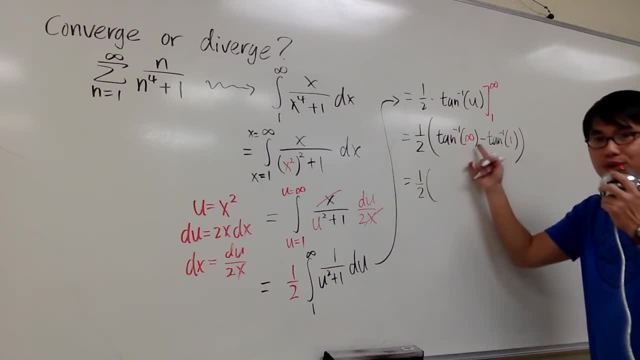 But then what's inverse tangent when u goes to infinity? This, right here, is pi over 2.. Okay, And then minus. And what's inverse tangent of 1? This, right here, is pi over 4.. And, as we can see, we have 1 half times pi over 2, minus pi over 4.. 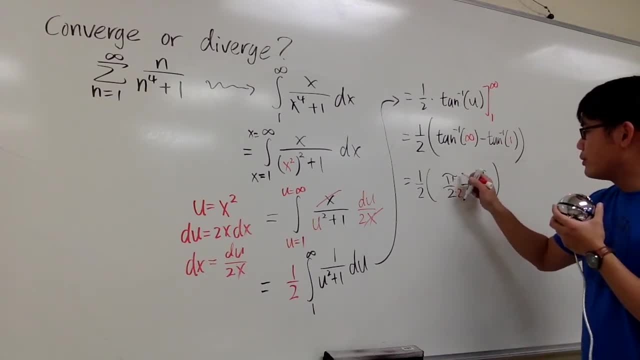 You can go ahead and do more. You can go ahead and say: multiply by 2,, multiply by 2.. Get the common denominator And then do this as 1 half times. This is just 2 pi minus pi on the top, which is just pi. 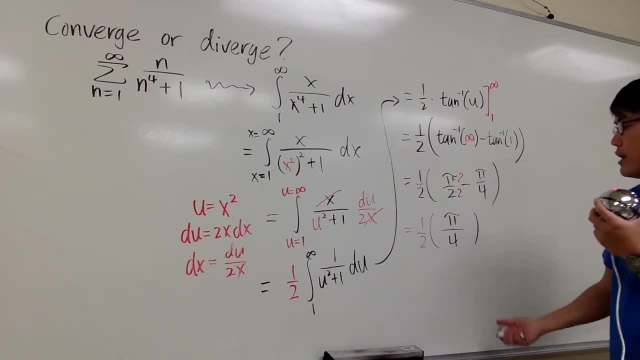 Over. this is the same denominator, which is 4.. Right, And then all this is just pi over 2 times 4 on the bottom, pi over 8. And all we're doing is just to show that this improper integral will give us a finite result. 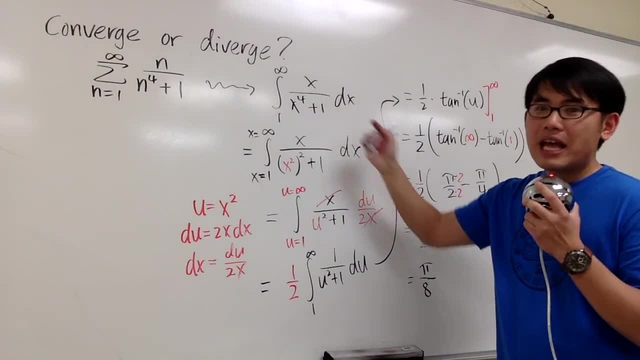 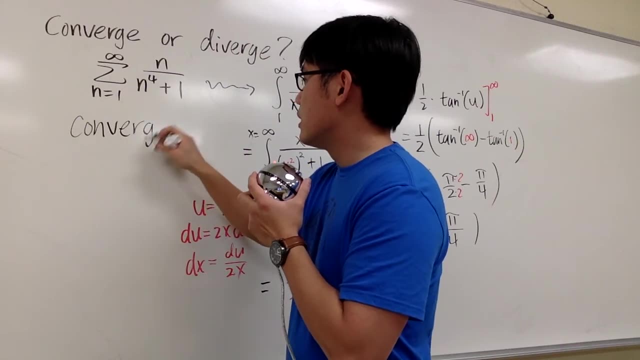 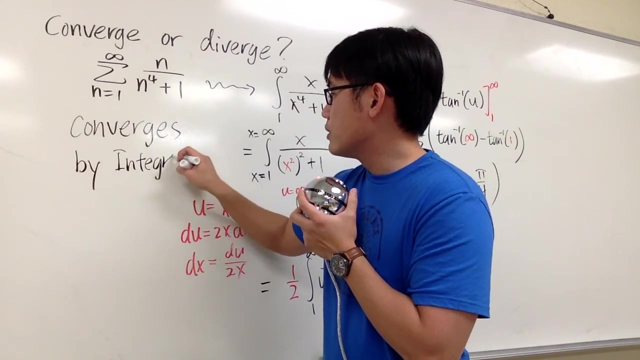 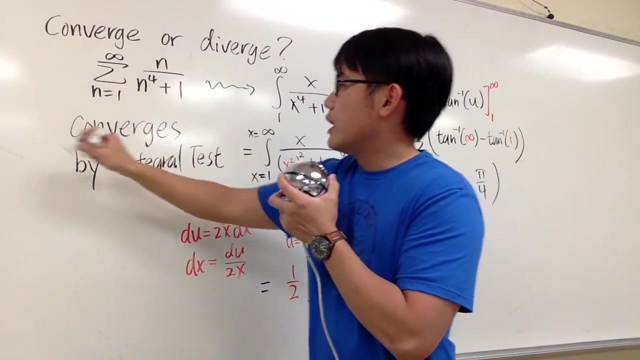 Namely this improper integral converges. Therefore, we get to say that this infinite series, it converges as well. Right, And the reason for that is by Integral test. Okay, So that's it. This infinite series- I should say the word- also converges by integral test. 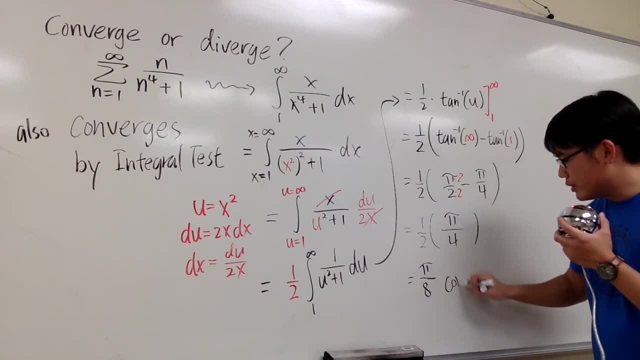 Because this integral, we get a finite number, which it was a convergent, That's it.